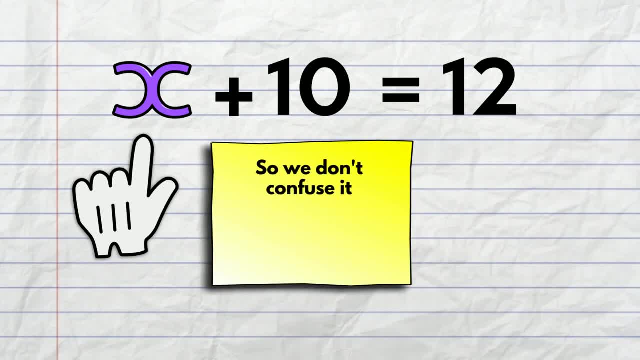 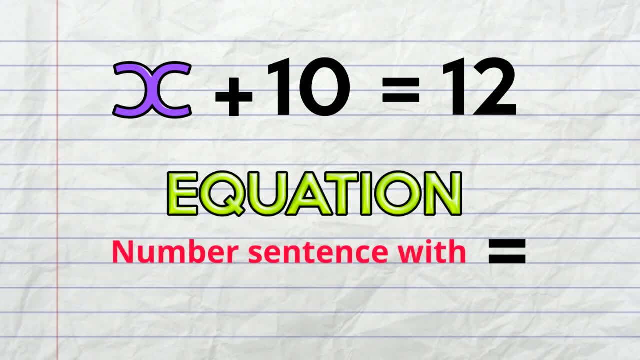 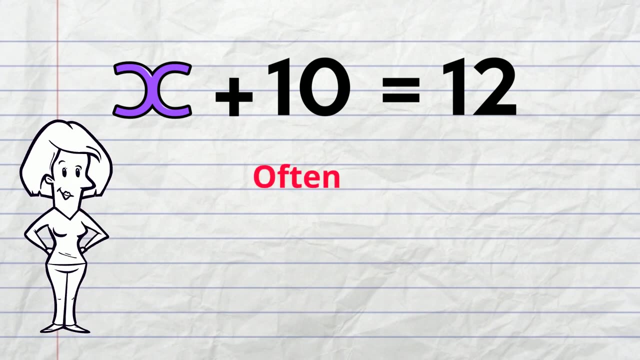 It's a curly kind of X, so we don't confuse it with the multiplication sign. Remember, equation is just the math word for number sentence with an equals sign. Algebra uses a letter, and it's often X or Y to stand for the unknown amount we're trying to find. 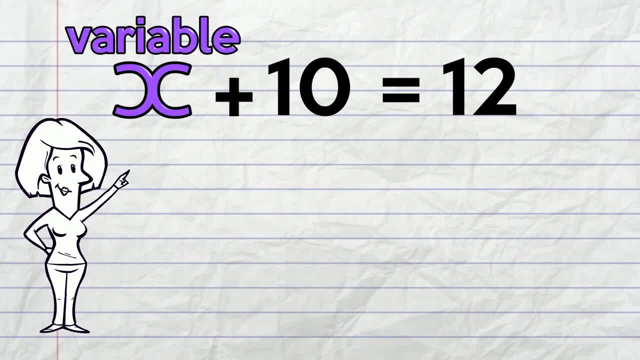 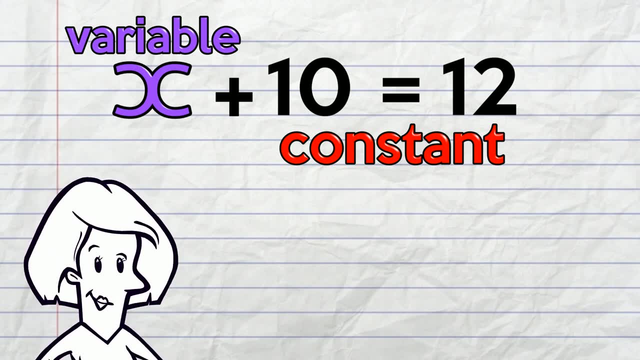 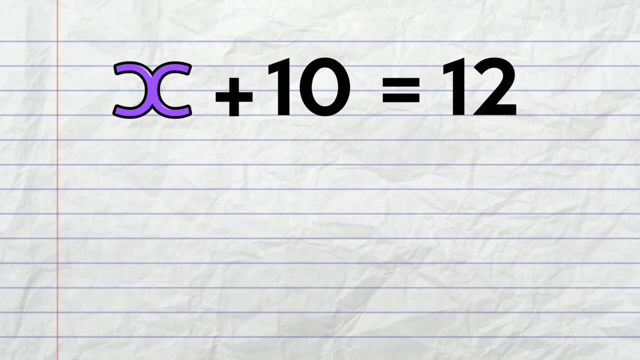 That unknown amount is called a VARIABLE. Any number value, like you see here, is called a CONSTANT. You need to know these math words and be able to use them. Of course, you can just count on from 10 to 12 and discover that X is 2.. 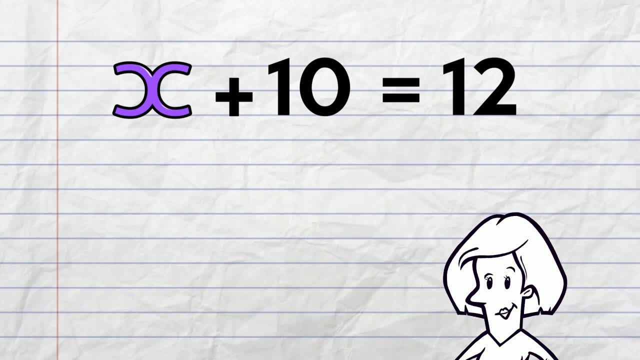 But we're going to do something a bit different. We're going to use a method that will work for any numbers. in any similar question, The goal in Algebra is to isolate the variable from the constants. This means we want X on one side of the equation. 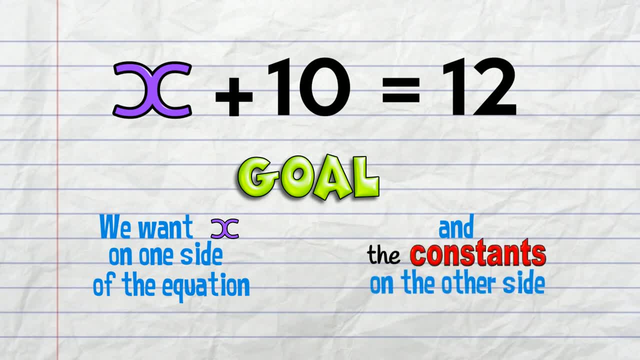 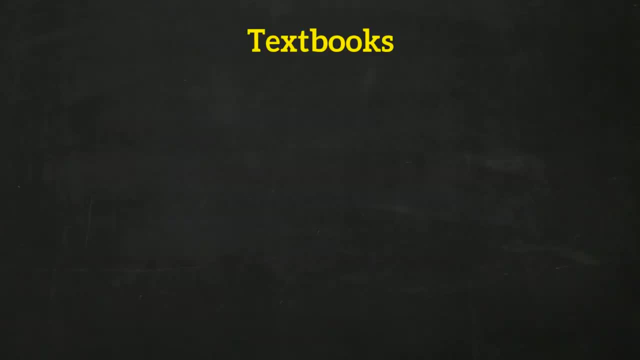 and all the numbers, the constants. on the other, We want it to say: X equals something. In textbooks they usually tell you to consider it as a balancing act. You can make changes to one side of the equation. That's one side of the equation. 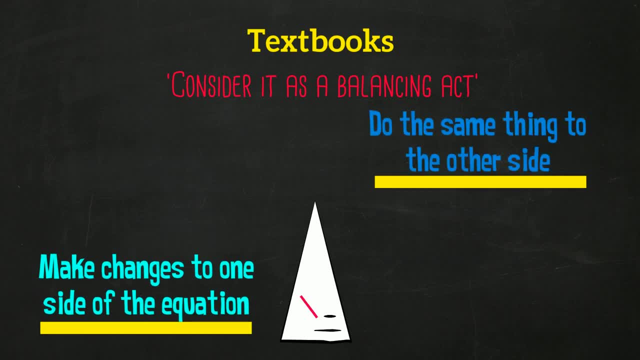 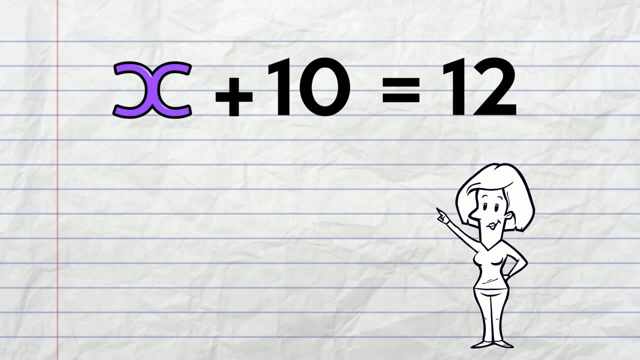 That's one side of the equal sign. As long as you do the same thing to the other side of the equal sign at the same time. Here I want to get rid of this 10 to get X on its own. I'm going to put minus 10 after it. 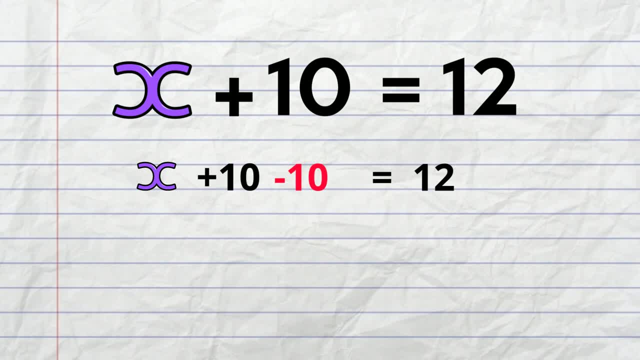 When I subtract 10 on this side, I have to subtract 10 on the other side of the equal sign too. I make this same change to both sides of the equation on this line of math, so it's balanced. On the next line, you can see we get. 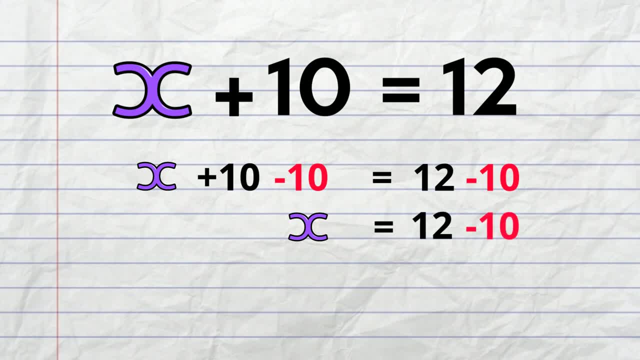 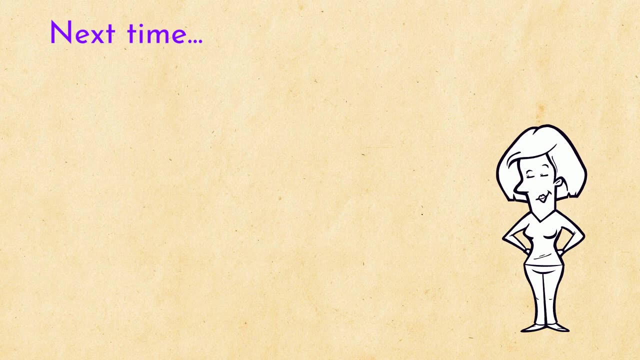 X equals 12 minus 10.. X is 2.. It's a straightforward approach. Whatever you do to one side, you must do to the other. Practice this method and see how it goes for you. Next time I'll show you.